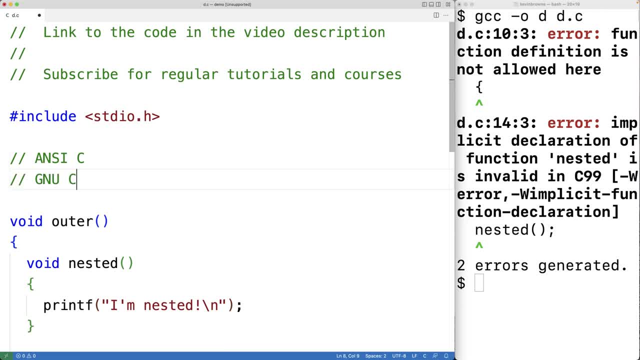 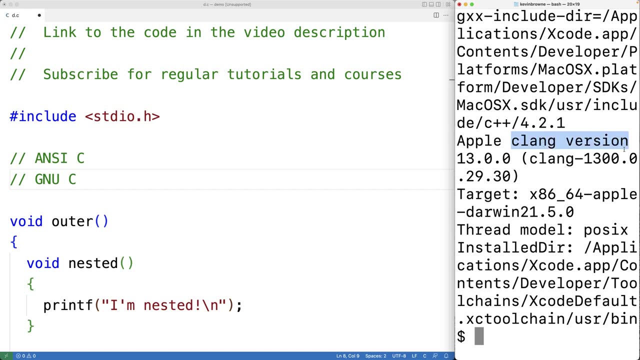 So GNU C, G-N-U-C does support nested functions. Now my machine is an Apple running OSX And if I check the compiler version with GCC-V, I see that my machine has the C-lang compiler installed, So it's not the GNU C compiler. 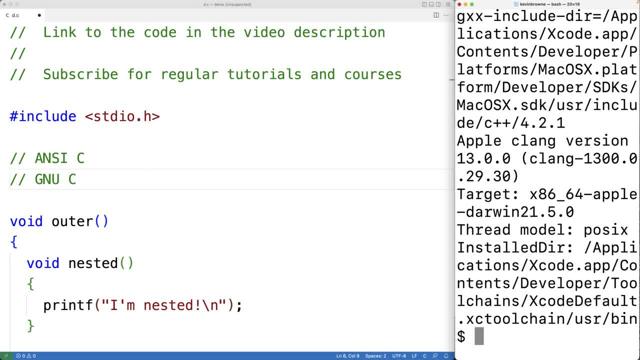 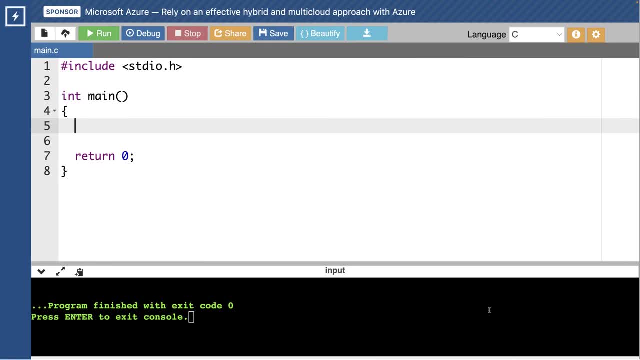 So that's why nested functions are not working with my compiler. Let's switch to an online compiler that does use GNU C. So this online compiler: here, I tested it out and it does use GNU C. So again, we'll make a function called outer, And inside the outer function we'll define a function called. 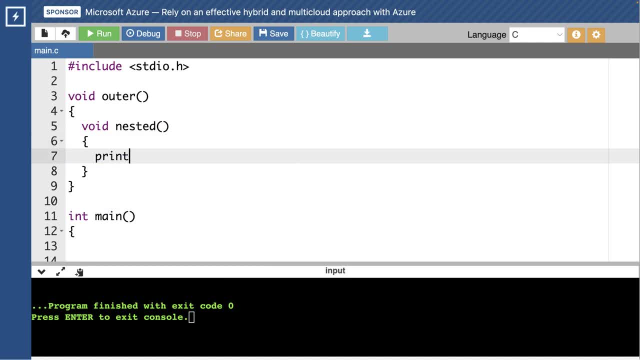 nested And the nested function we'll again just print out I'm nested, exclamation mark and followed by a new line, And then we'll call the nested function from within the outer function. Then in our main function we'll call outer And if we run our program, 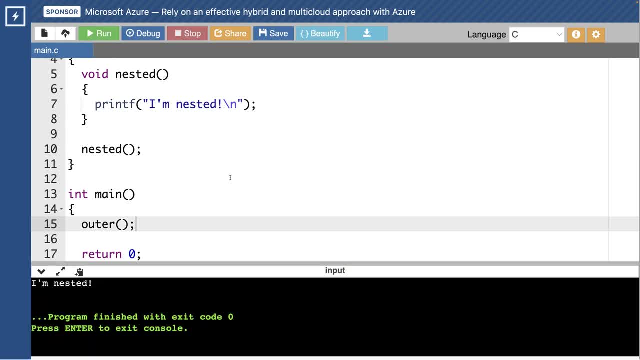 this time it's going to work. We get the output. I'm nested, And that's because this online compiler does use a GNU C compiler on the backend. A nested function can actually access a local variable of its containing function so long as that variable is visible when the nested function is defined. 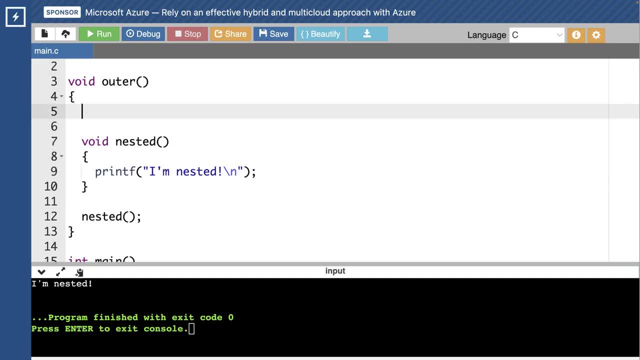 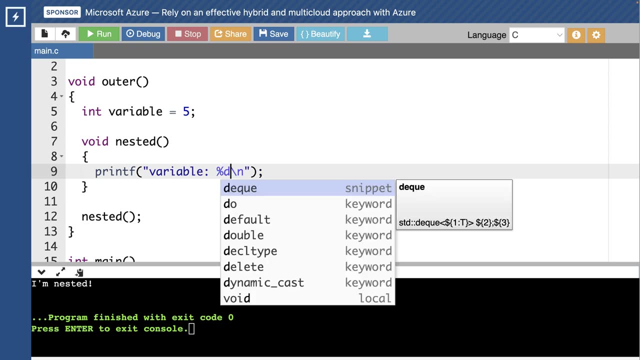 So for example, in our containing function outer we could declare a variable called variable. that's going to be an int And we'll assign a variable, the value five. The nested function could actually access this variable. So we'll have variable colon percent d backslash n And we'll actually access and output the variable value. 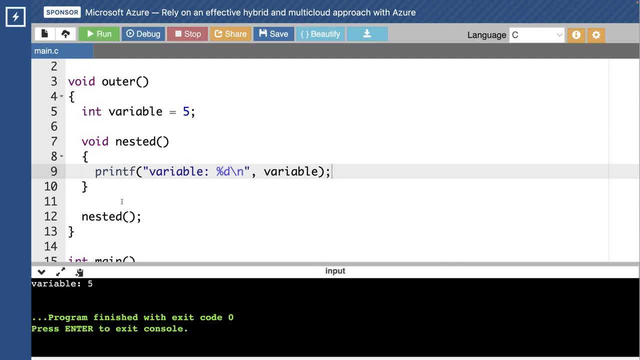 We can run this program and we get variable colon five, So we actually can access the local variable of the containing function. The variable does have to be visible, though, when the nested function is defined. So, for example, if we declared a variable here called 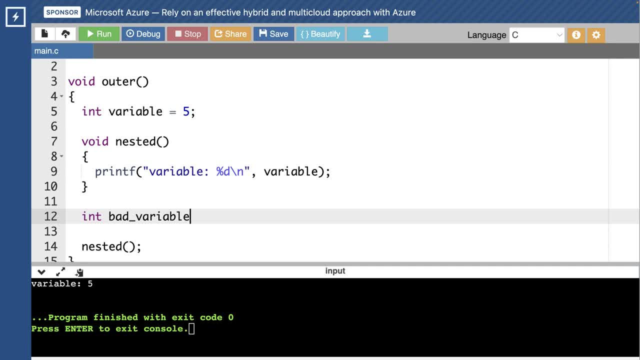 bad underscore variable. this variable is not going to be visible to the nested function when it's defined. So if in our nested function we try to access bad variable, it's not going to work. So here we'll have printf, And this time we'll have bad underscore variable. 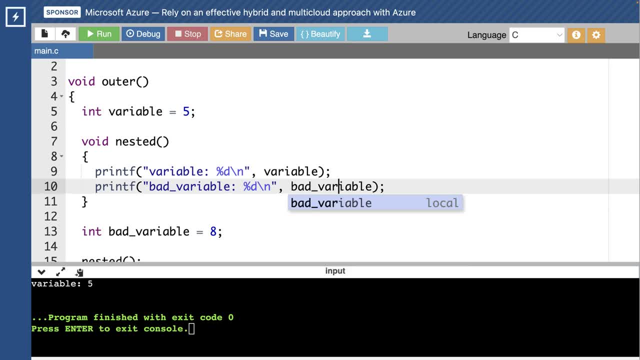 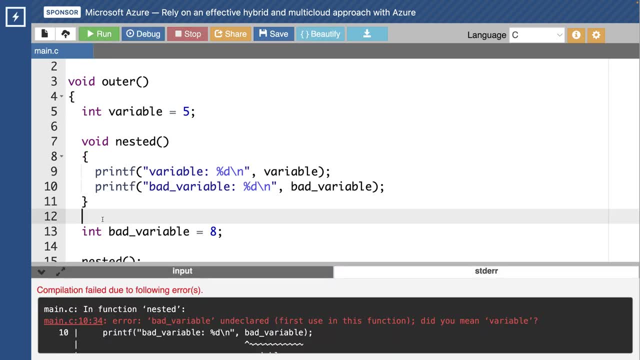 And we'll try to output bad underscore variable. And then if we run this program we get this compiler error here It says bad variable undeclared. So that is one restriction on using the containing functions local variables, One reason why it could be a. 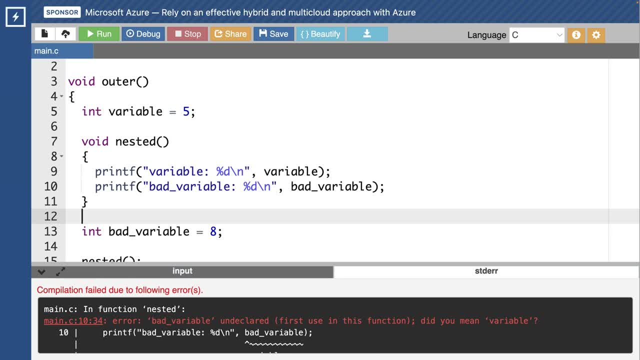 good idea to use a nested function is that it allows us to access the local variables of the containing function. When we access the local variable of the containing function, it saves us from having to pass the value as an argument to the nested function. If a nested function has another parameter, that's going to take up space on the stack. 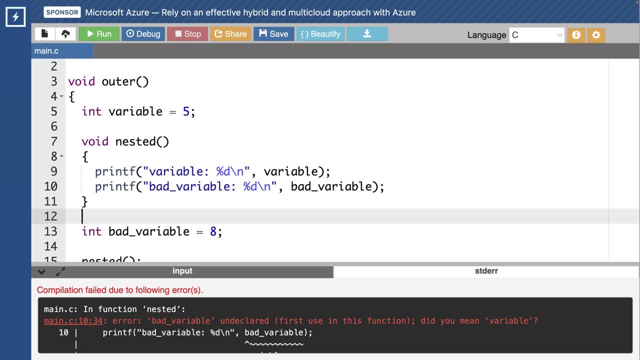 each time we call the function. By using the containing functions local variable directly, we're saving that space, And if our program is running on something like an embedded system, that might actually be important. So I should also note that we can't call a nested function until 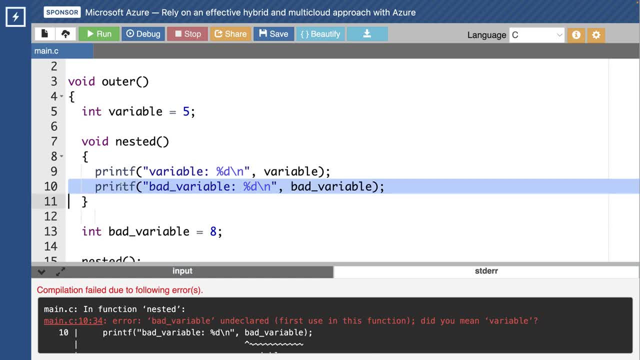 it's been declared or defined. So I'll delete these lines here that caused this error And then I'll try to call the function nested up here before it's been defined or declared. When we run the program we'll get a different compilation error here. 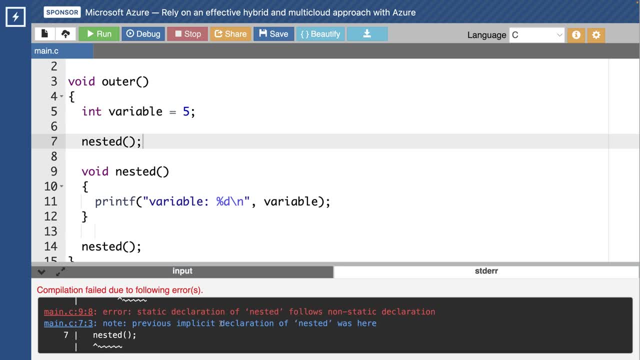 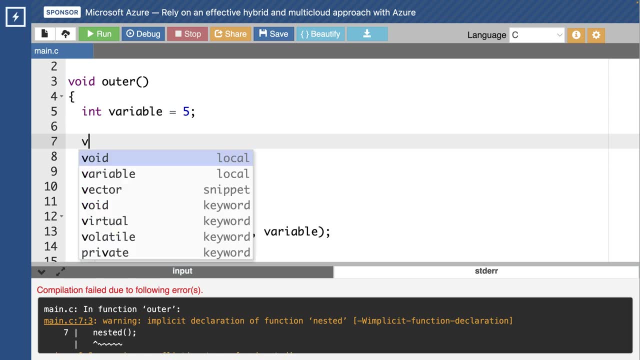 It says error: static declaration of nested follows non-static declaration, So we can't use nested like this. We could try to declare nested above where we call it like this: void nested, And that is how we would normally declare a function. But if we try to run this, 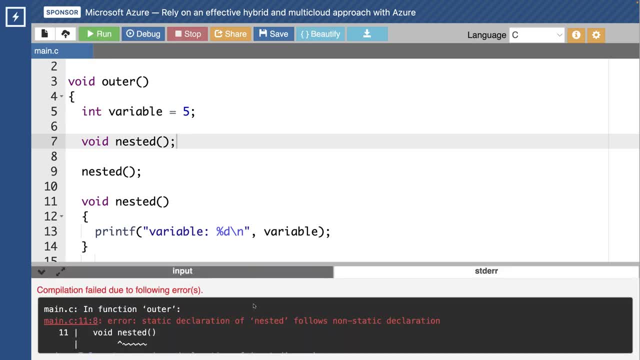 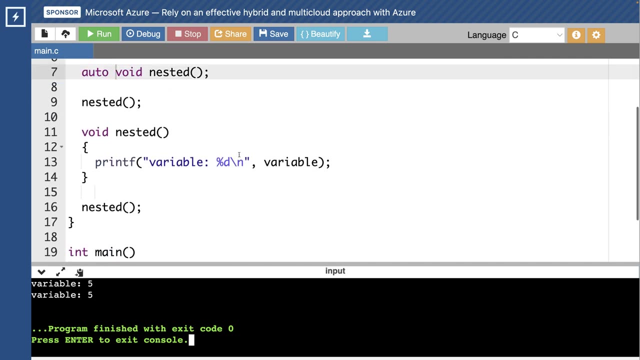 we'll also get an error. So we also get an error here, And this here is pretty interesting. To make this work, we have to use the auto keyword here like this: Then if we compile and run our program it will actually work. We call the nested function twice Once here, above where it's defined. 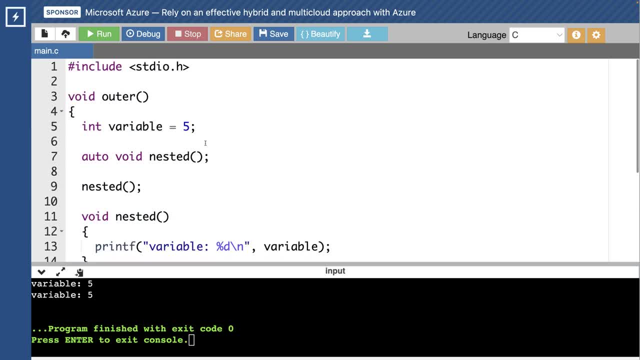 and once here below where it's defined. And that's okay, because here we first declared the function. and the reason why I say this is interesting is that the auto keyword is normally pretty useless in C. So C has different storage classes, like extern and static, that affect the lifetime and 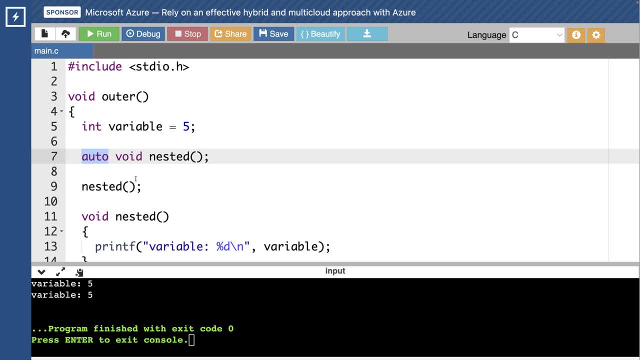 scope of a variable, among other things, And the auto keyword is for the automatic storage class. It's the same storage class that is used by default when we declare a variable like this inside a function. It's the storage class that's there when we don't actually specify a storage class. So it's just kind of interesting, because normally 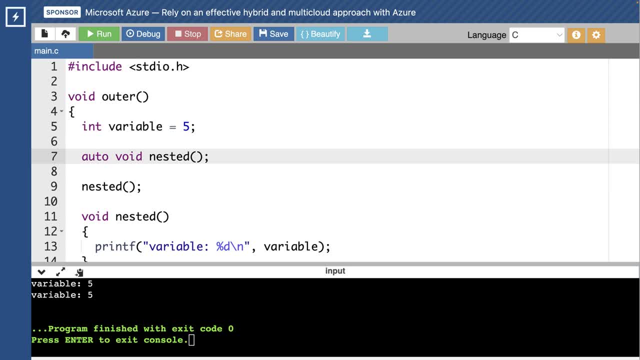 the auto keyword doesn't do anything useful at all, But in this case here, it's actually necessary to use it. Another reason why we might use nested functions is if we want to make it very clear that the nested function belongs to the containing function, in the sense that the nested function 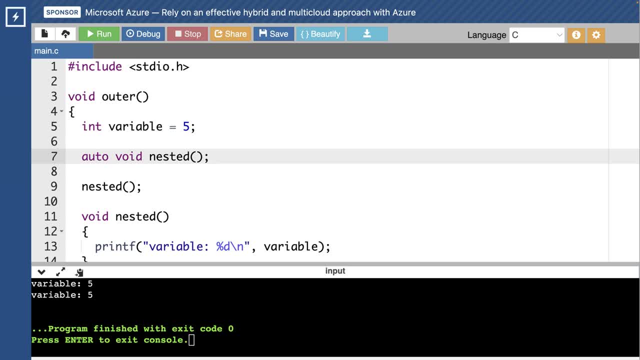 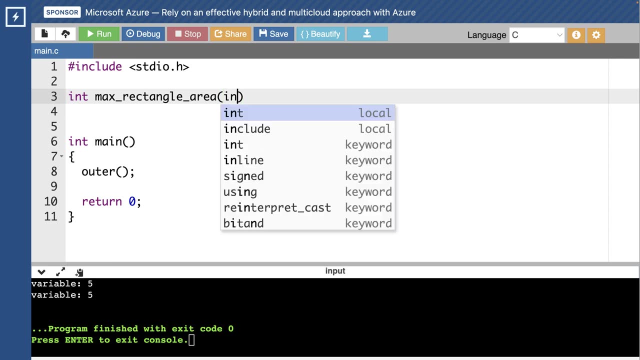 should really only be used within the containing function. So, for example, we could make a function to find the largest rectangle area. We'll call the function int max rectangle area and the function will accept four parameters: The width of the first rectangle. the length of the first rectangle. 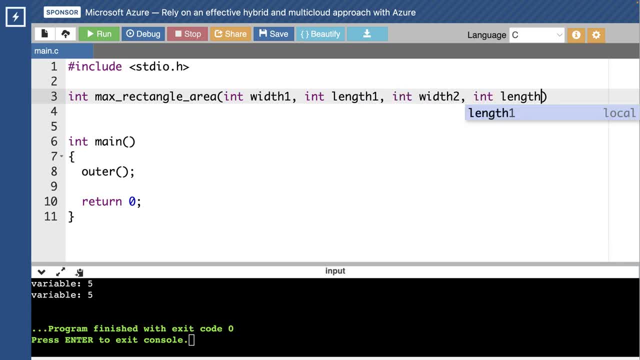 the width of the second rectangle and the length of the second rectangle. And inside the max rectangle function we can make a function that can only be used within the container function. We'll define a function called rectangle area that's going to calculate the area of a rectangle. 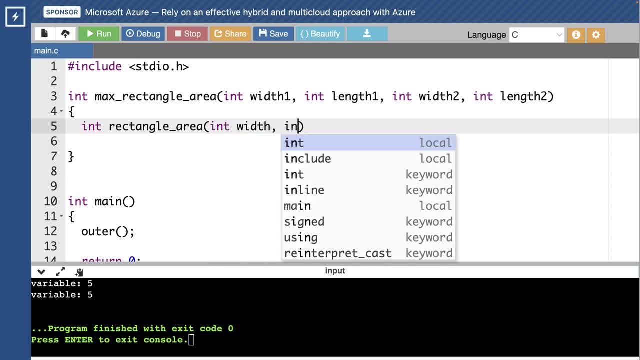 So this function will have two parameters, width and length, and the function is going to return width times length to calculate the rectangle area. Then we can calculate the area of rectangle one using this function and we could pass it width one and length one. Then we could calculate the area of the second rectangle with. 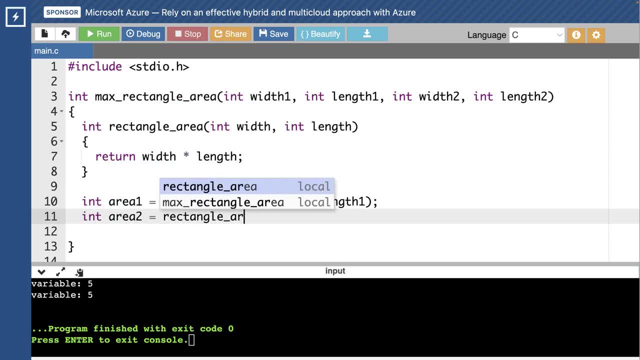 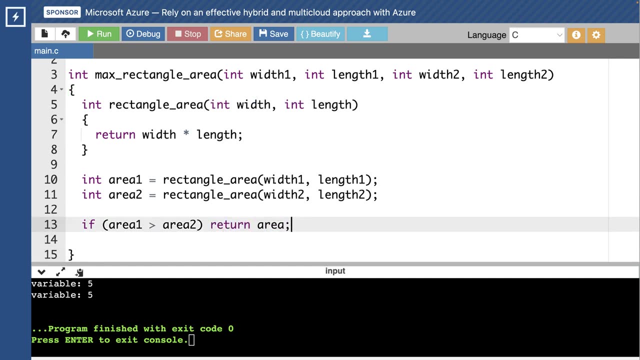 int first, rectangle and length. one int area2 is equal to rectangle underscore area and we'll pass it width2 and length2.. Then we could return which area is bigger. So if area1 is greater than area2, we could return area1.. 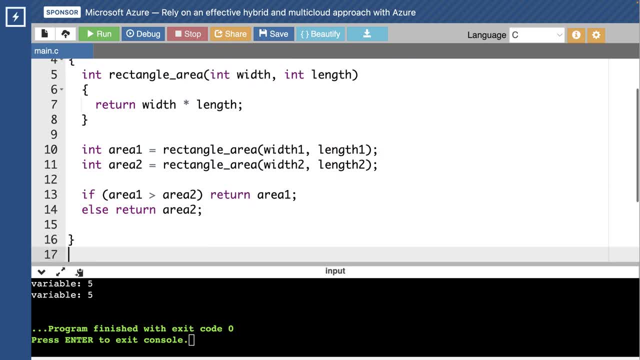 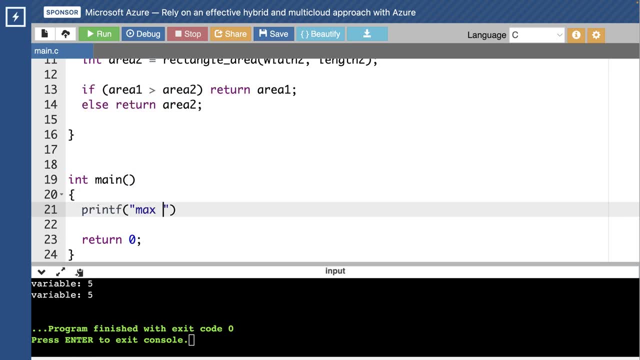 Otherwise we could return area2.. Then we could call our maxRectangleArea function. So down here we could say: printf: maxarea, colon %d, backslash n, and then we'll call maxRectangleArea and we'll pass it some different rectangle dimensions like 4 and.